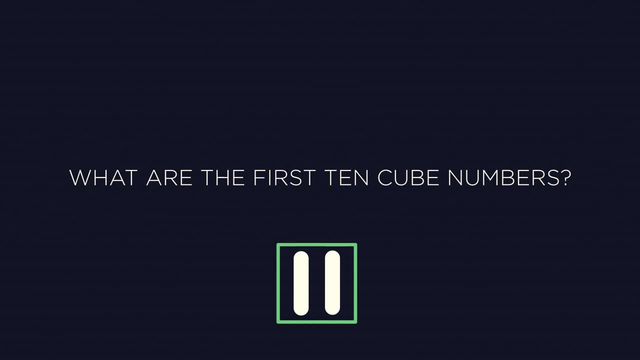 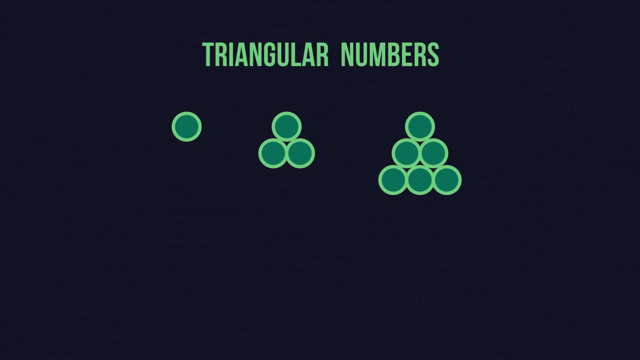 Pause the video and have a go. How did you do? Our final look is at triangular numbers. A triangle number is the number of objects you can arrange in a perfectly filled equilateral triangle. Another way to look at this is: each time you increase the number, you increase the. 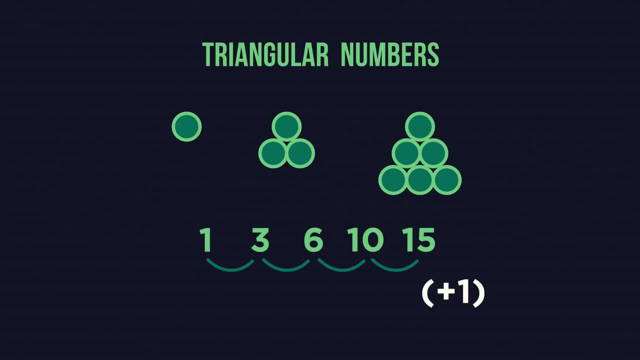 previous gap by one. One to three has a gap of two, Three to six has a gap of three, Six to ten has a gap of four, and so on. You can imagine this by stacking equilateral triangles. For example, the first triangular number is one with the row of triangles. 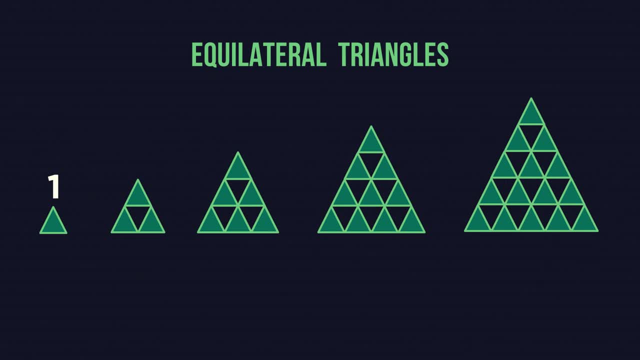 The second triangle has a row of triangles. The third triangle has a row of triangles. The third triangle has two rows, giving three triangles. The third number needs three rows, so gives six triangles, and so on. See if you can work out the remaining first 10 triangular numbers. 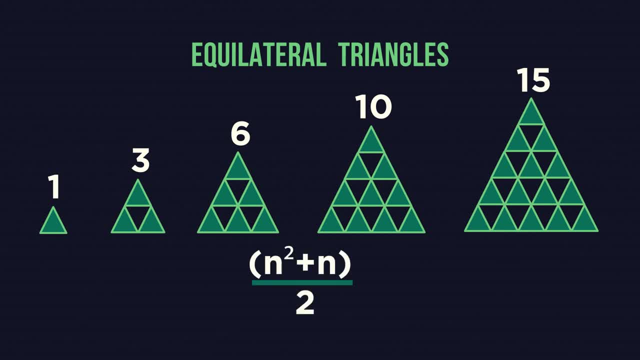 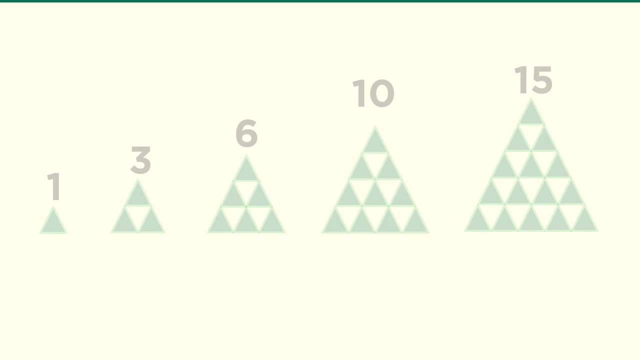 The nth term for finding a triangular number is n to the power of 2 plus n divided by 2.. You can find this if you look at the equation for the Euler theorem: quadratic sequence. See this video here for more information. Now for the clever bit. If you look carefully, between the coloured triangles are white triangles. 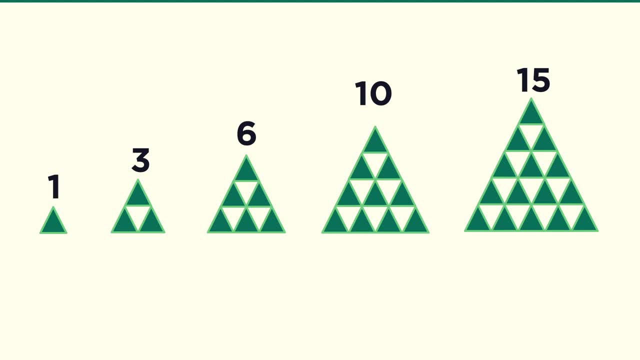 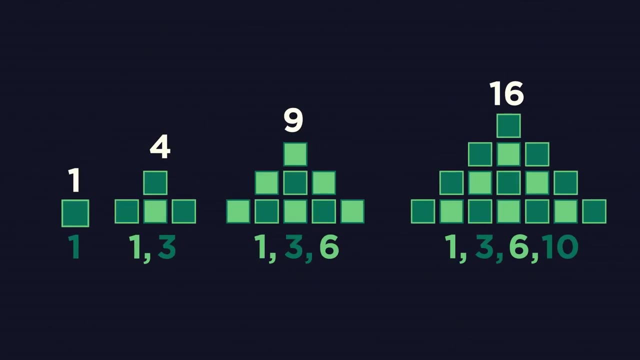 the opposite way round. If you count all these triangles, you get another sequence of numbers 1,, 4,, 9, 16.. Familiar, Yes, these are square numbers. again, You can also see triangle and square numbers together in this pattern If you count alternating colours. exactly. 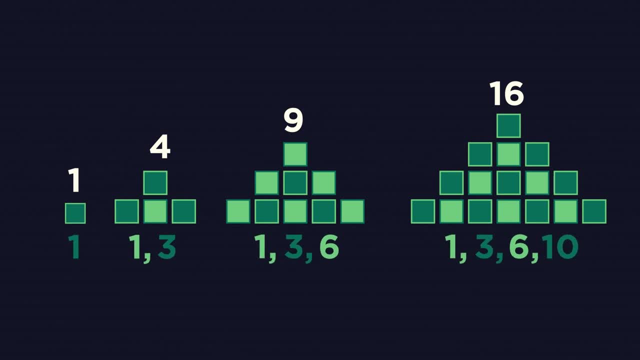 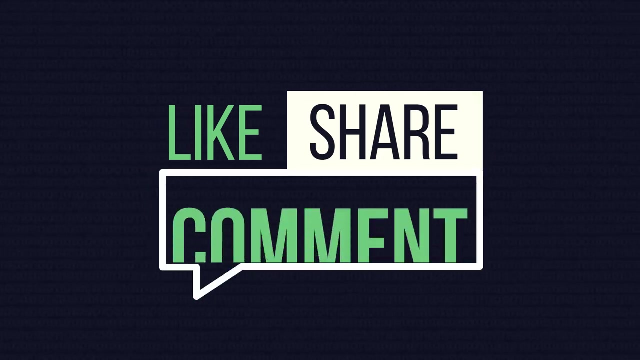 you get triangular numbers. If you count the total, you guessed it square numbers. So there you have the basics of square, cube and triangular numbers. Please like and share our videos with your friends. If you have any questions that you want help with, just comment below. Subtitles by the Amaraorg community.